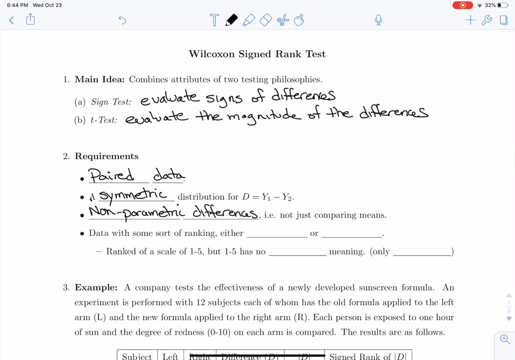 So this is comparing data with some sort of ranking, either cardinal or ordinal. An example would be to rank something like, say, course evaluations on a scale from 1 to 5.. But the numbers 1 through 5 have no absolute meaning, only a relative meaning. 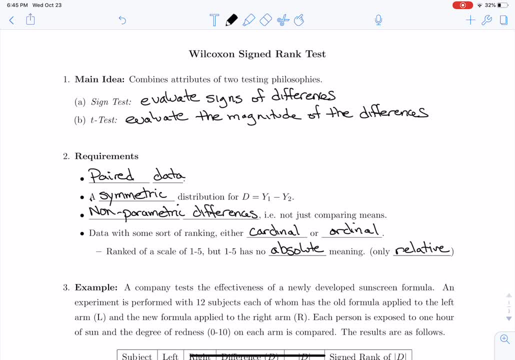 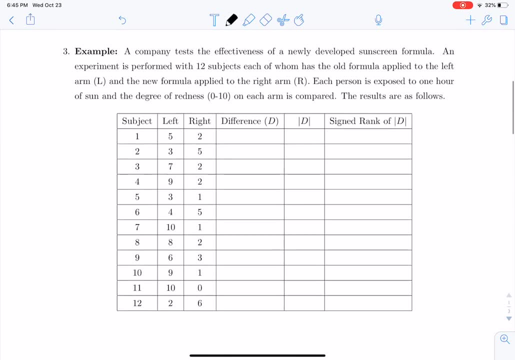 That 5 is bigger than 4, is bigger than 3, bigger than 2, bigger than 1.. So we're going to move on to an example, and this example is going to be similar to the one I just showed you. 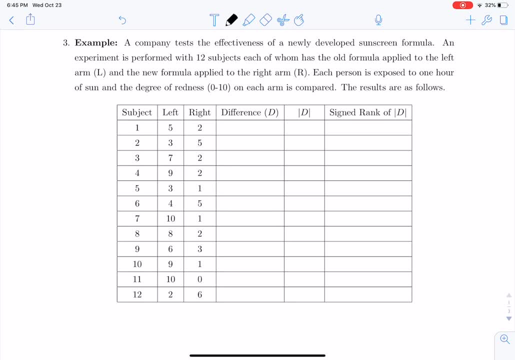 This is going to be similar to the one that we did for the signed test. Here again, a company is going to test the effectiveness of a newly developed sunscreen formula, and they're going to perform an experiment with 12 subjects, not 25 like the signed test. 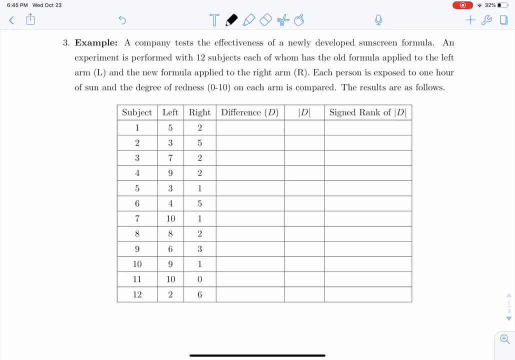 And each of them has the old formula of sunscreen applied to the left arm and the new formula of sunscreen applied to the right arm, And then, for each one, each person is exposed to one hour of sun, and the degree of the sun is different. 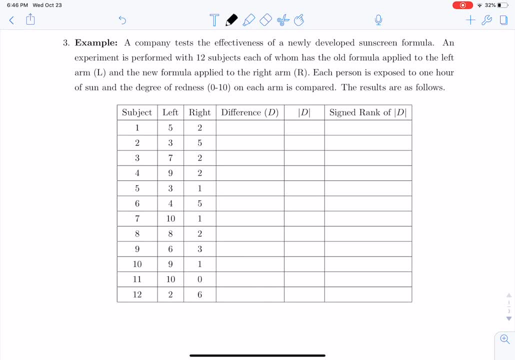 The degree of redness on a scale from 0 to 10 on each arm is compared. So with the signed test we just looked if the left arm was more red than the right arm or vice versa. But here we're going to assign a numerical score between 0 and 10 to determine the degree. 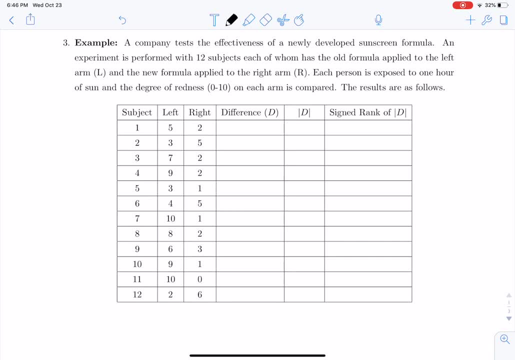 of redness on each arm. Now, that numerical scale from 0 to 10 is not a measurement, not like when we're measuring heights and weights and things like that. It is just a numerical scale that we're assigning to the redness. 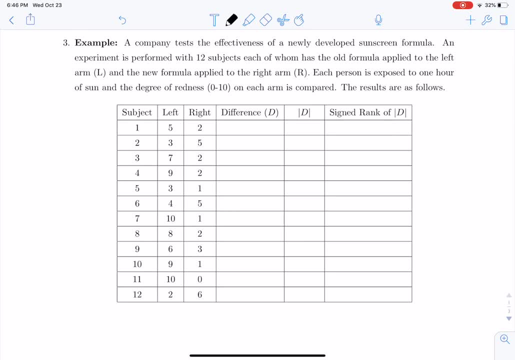 And so the numbers 0 through 10 don't have any meaning other than the fact that 10 is more red than 9, is more red than 8,, et cetera, et cetera. The first thing that we will have to do in order to apply the Wilcoxon signed rank test is: 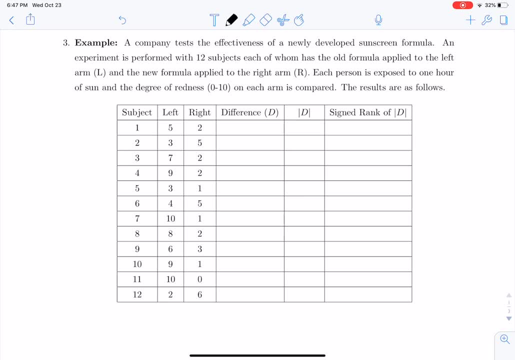 to calculate the differences in the scales between the left arm and the right arm. So for the first subject, we saw that the left arm had a redness score of 5, and the right arm had a redness score of 2. And so the difference was 3.. 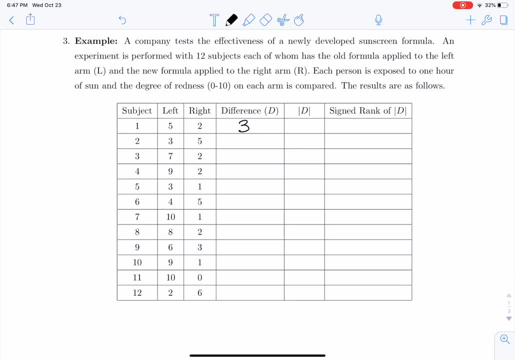 The second subject, the left arm had a redness of 3, and the right arm had a redness of 5,, so the difference is negative 2.. And then we can keep computing the differences. The difference is all the way down. 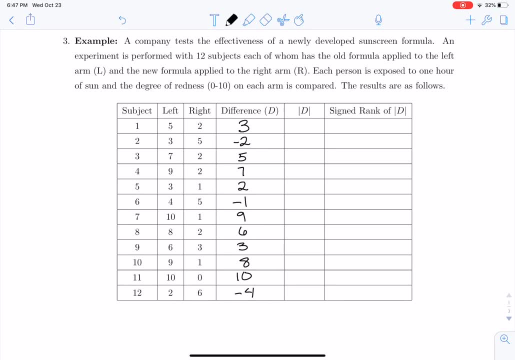 Now we're going to want to look at the absolute values of these differences to see how big they are. So here I'm going to take the absolute value of each one of the differences And then we're going to look at these differences and we're going to look at the absolute value of each one of the differences. 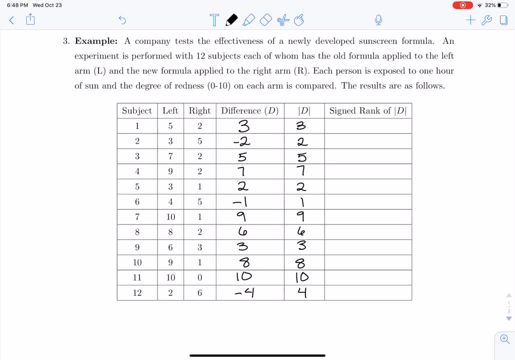 And we're going to rank them from 1 to 12.. 12 being the largest difference and 1 being the smallest difference. So we notice that subject 11 has the largest difference of 10, so we give that a rank of 12.. 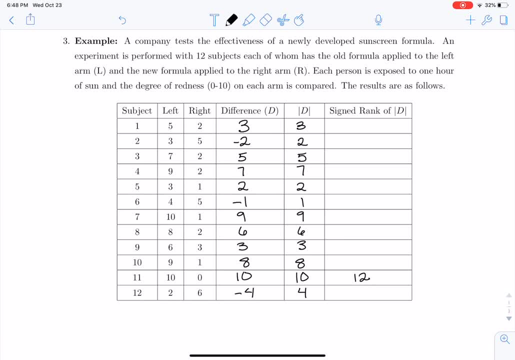 Subject 7 has the next largest difference of 9, so we give that a rank of 11.. Subject 10 has a rank of 10. Subject 10.. Subject 4 has a difference of 7, we're going to rank that 9.. 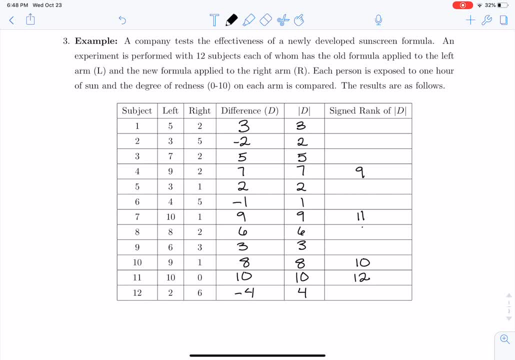 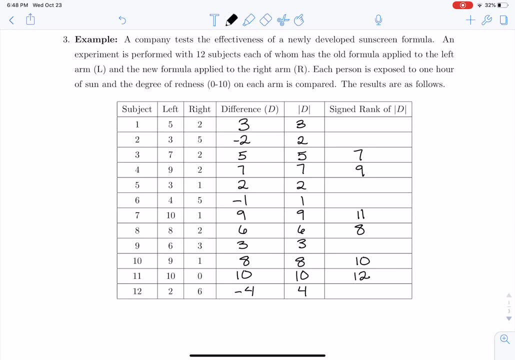 Subject 8 is going to have a ranking of 8.. Subject 3 is going to have a ranking of 7, because 5 is the next largest number And then the next largest from 5 is going to be 4.. That's going to have a ranking of negative 6.. 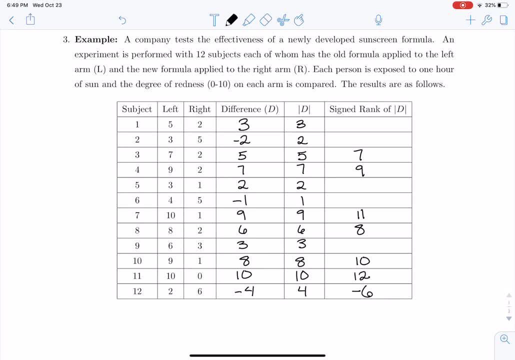 And then the next largest is 3, and we notice that 3 actually appears twice. So the difference of 3 appears here once and here once. So the way that we deal with that is that we assign the next largest ranking of 5 to one of the 3's. 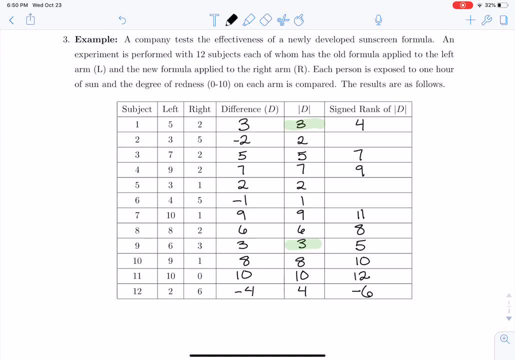 and the next largest ranking, of 4 to the next 3.. And then we're going to want to average those two rankings of four and five. So we're going to average this number and this number. So the average of four and five is four and a half. 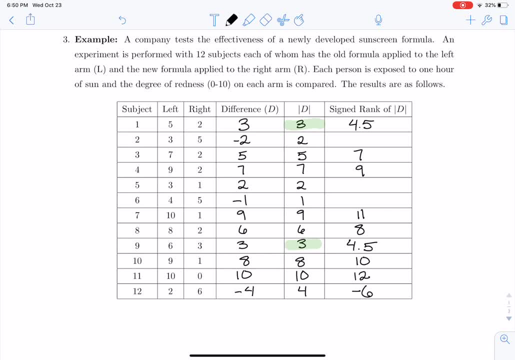 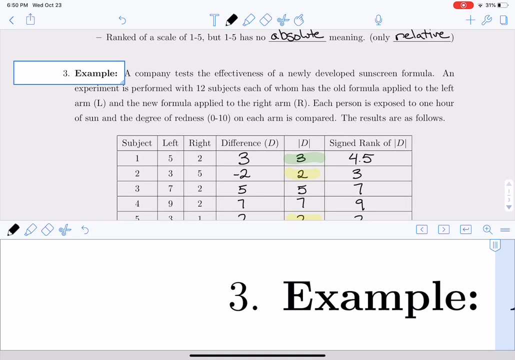 Now the next largest difference is going to be two. You'll see that one of the twos is positive and one of the twos is negative. The rankings for those twos would normally be three and two, but we're going to average them. 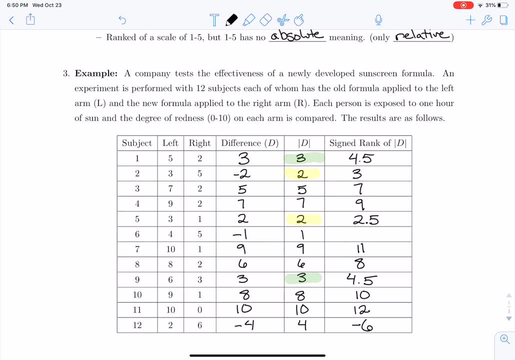 so that we get two and a half for one of the twos and two and a half for the other two, And then we're going to average that, And then we're going to average that, And then, finally, the smallest difference is one, and that gets a ranking of one. 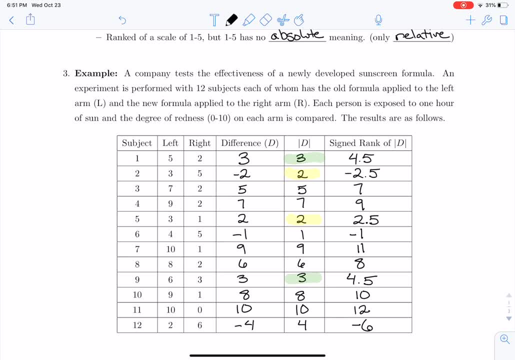 Now notice that I've put negative signs in front of the rankings for the negative differences. So here we can see there's a negative sign for subject two because there's a negative difference there. There's a negative sign for subject six because there's a negative difference there. 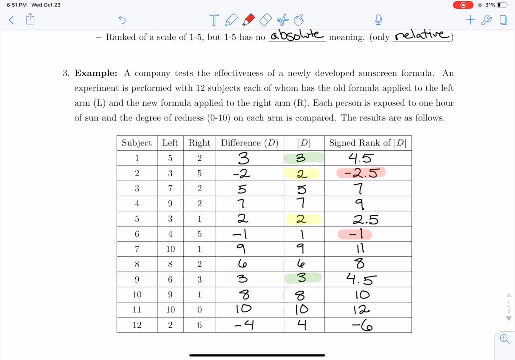 And there's a negative sign for subject 12.. And there's a negative sign for subject 12 because there's a negative difference there. What's important to realize is that the numbers I've computed in the right most column are not the differences. 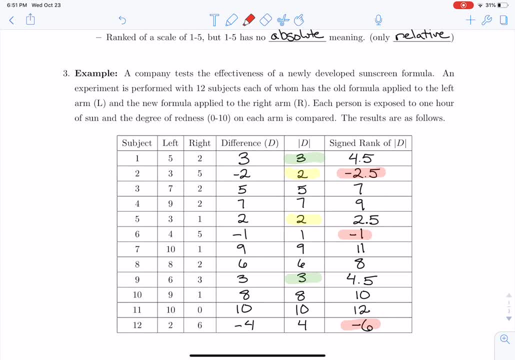 but the rankings of the differences. So you should see all of the numbers represented, starting with one- two. but two isn't there because it was a tie. So I have one, two and a half And two and a half, And then, because threes were tied, the differences of three were tied. then I had four and a half and four and a half. 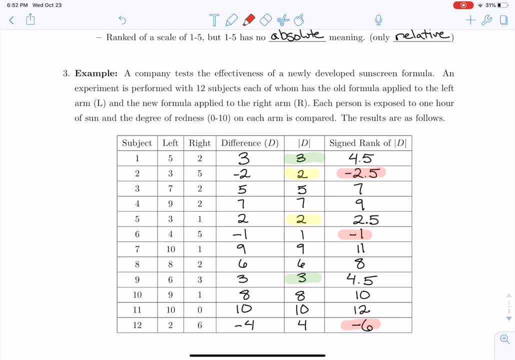 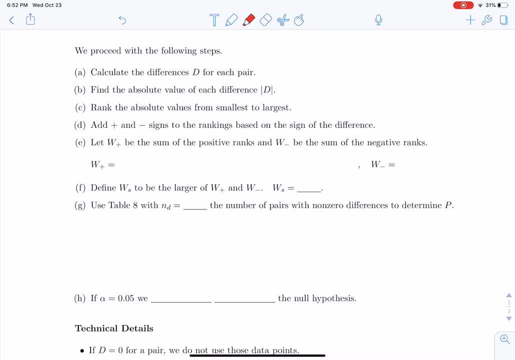 And then, finally, I start with six, seven, eight, nine, ten, eleven and twelve. Okay, so what are we going to do with these numbers? Well, we've already calculated the differences for each pair. We found the absolute values of the differences. 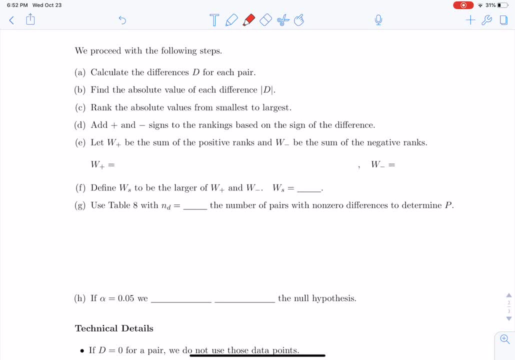 We rank the absolute values from smallest to largest. We added plus signs and minus signs to the rankings based on the sign of the difference, And now I'm going to compute two numbers: W plus will be the sum of the positive ranks and W minus will be the sum of the negative ranks. 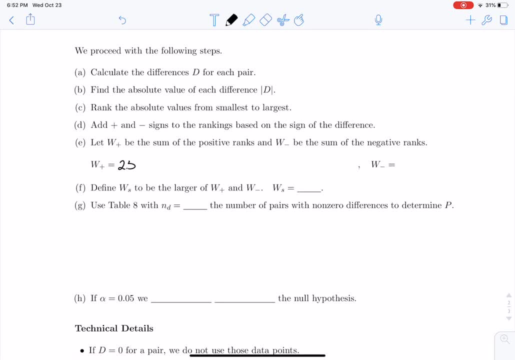 So, looking back at our data, our positive ranks were two and a half, Four and a half, four and a half, 5,, 7,, 8,, 9,, 10,, 11, and 12.. Our negative ranks were 1,, 2, 1⁄2, and 6.. 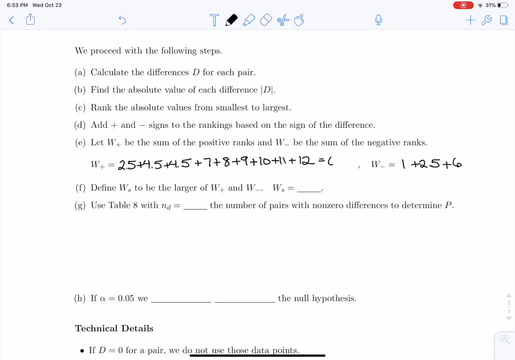 So the sum of all the positive ranks were 68 1⁄2, and the sum of all the negative ranks, in which I've removed the negative signs, were 9 1⁄2.. So the test statistic, much like the sign test, is going to be the larger of w plus and w minus. 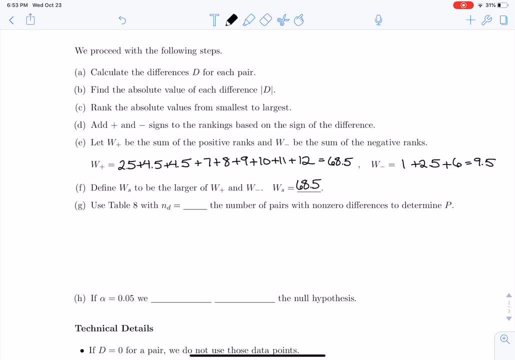 in this case 68 1⁄2.. And then we will need to refer to Table 8 in order to figure out the p-value here, where the number of differences, the number of subjects that we looked at, was 12.. So, with a test statistic of 68 1⁄2 and a number of subjects of 12,, 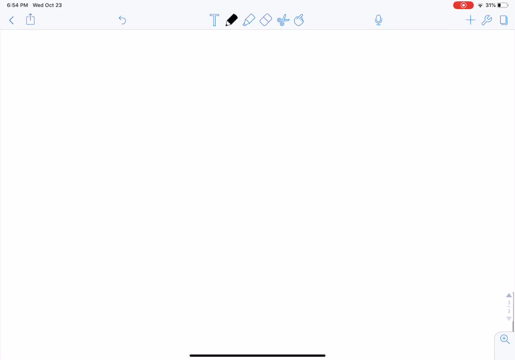 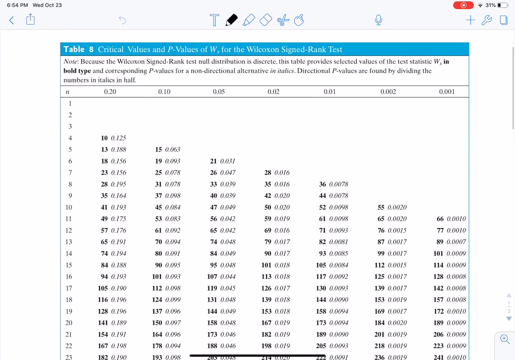 I'm going to go down to our table for the Wilcoxon rank test. Here we are And I'm going to highlight for a number of differences, number of differences being 12, 12 subjects and the number 68 1⁄2 would appear right here, between 65 and 69. 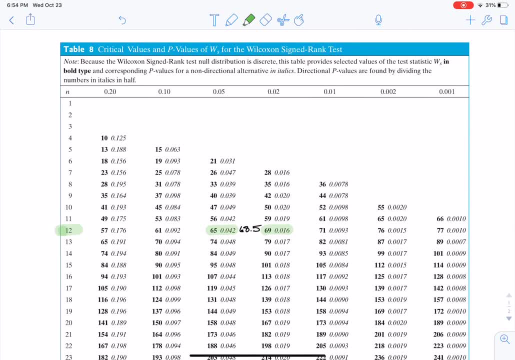 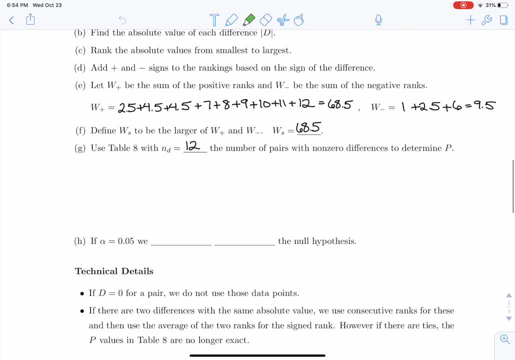 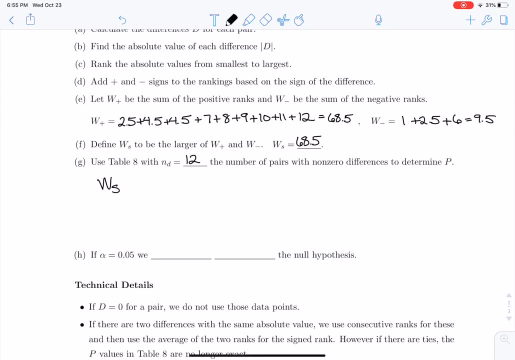 So let's look at our p-value. So let's look at our p-value. So let's look at our p-value here. Here, for Ws being 68, 1⁄2 and our number of differences being 12, we got that the p-value was between 0.16 and 0.042.. 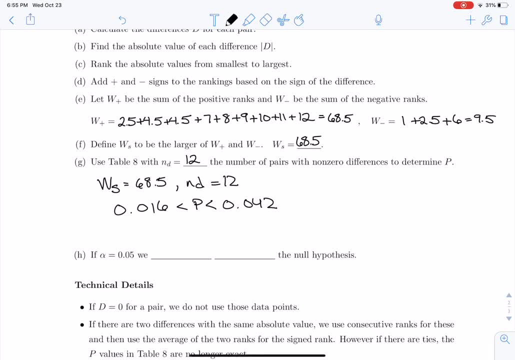 And if we use an alpha of 0.05, we can reject the null hypothesis. And so notice, by having some sort of scale of redness and looking at the differences of the degrees of redness for this test with only 12 subjects. 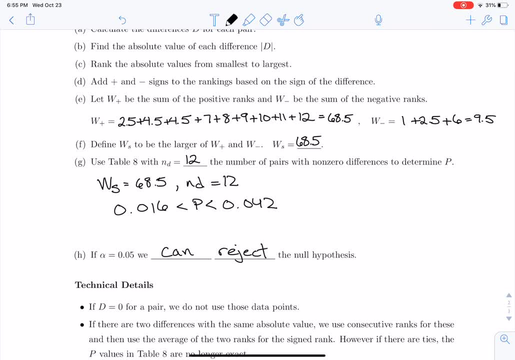 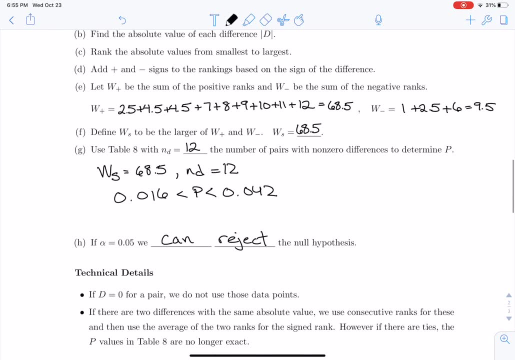 we were actually able to get statistical significance, Whereas with the sign test we were not able to do that with 20 subjects. So let's look at some tests. So let's look at some tests. So let's look at some technical details. 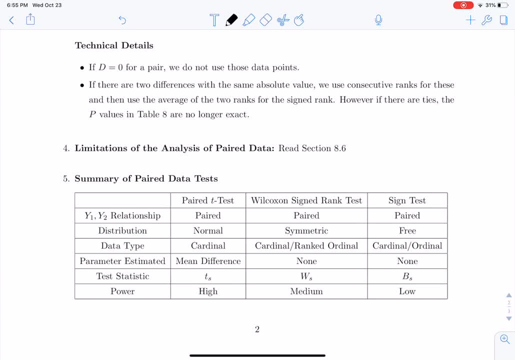 First, if the d equals 0 for a pair, then we do not use those data points. If there are two differences with the same absolute value, as I said before, we use consecutive ranks for these and then average the two ranks for that signed rank. 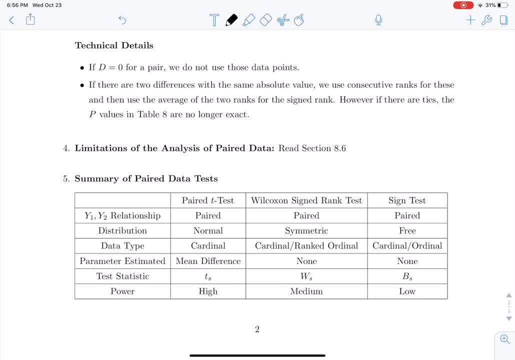 However, if there are ties, the p-values in table 8 are no longer exact. We should sum up, Summarize our discussion of paired data tests we looked at in chapter 8, the paired t-test, the Wilcoxon signed rank test and the signed test. 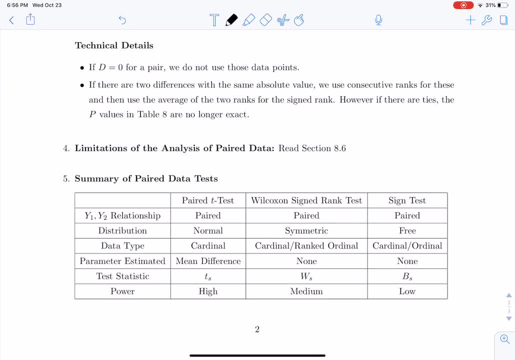 If you can do a paired t-test, that is the best situation. If you have a normal distribution and you're looking at the difference in means, then this is the highest powered test. If you don't have a normal distribution but you do have a symmetric distribution,